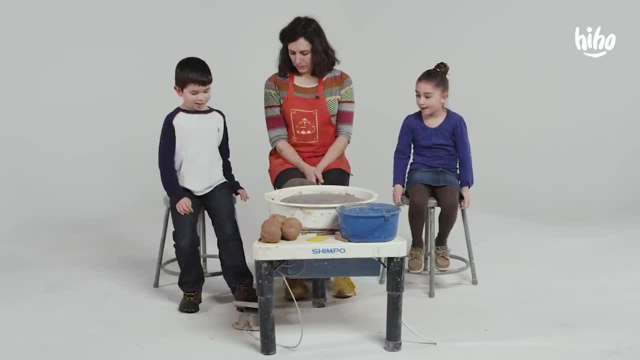 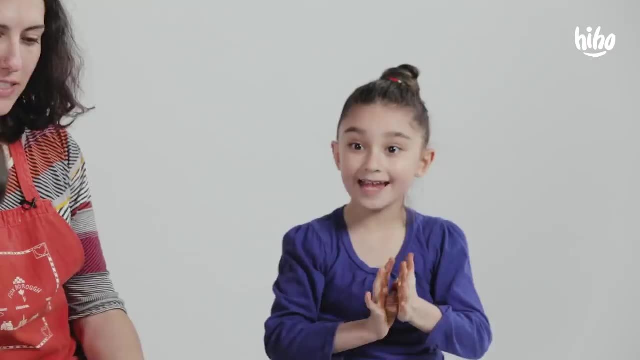 Wow, that's exciting. What do you think this is? I step on this and then, while that's spinning, we shape it out. Let's go to make a teapot or something I can make a doll. It's gonna be named Bon Bon. 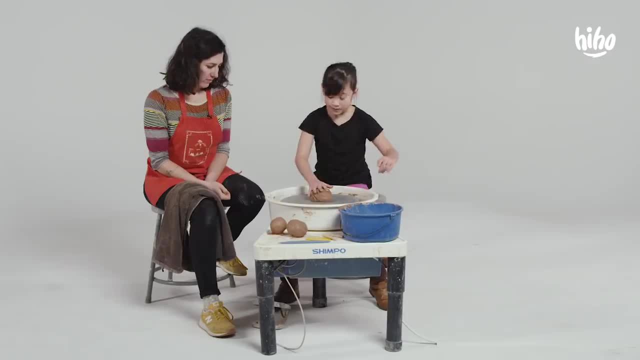 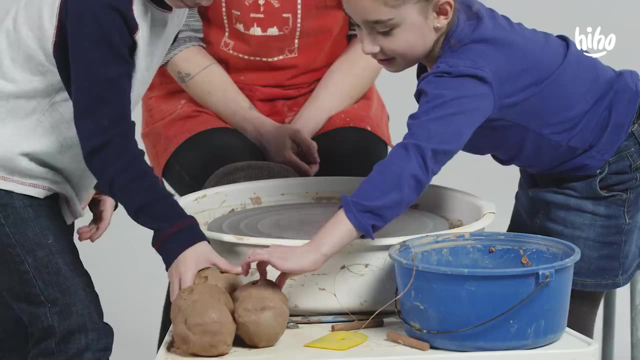 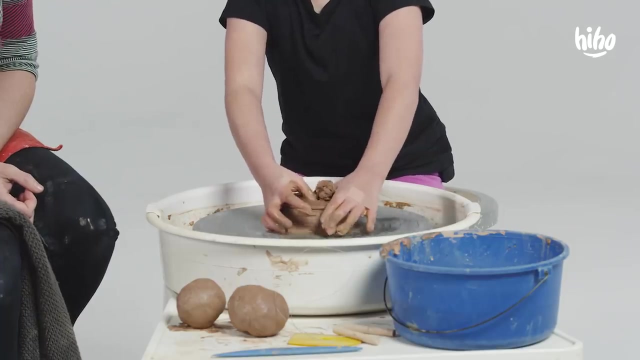 You wanna give it a shot? Sure, Okay, Perfect, I can touch that. Yeah, Sticky, Ew. It looks like you've done this before. I never actually did this before. Whoa, Can I do it? Um? 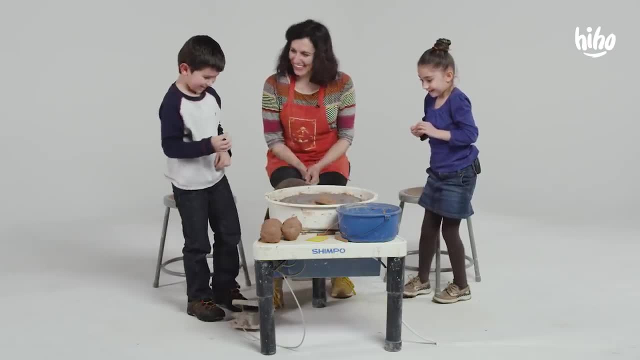 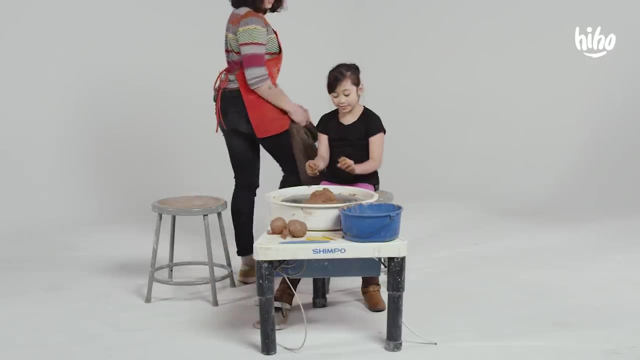 Here. let's stop it. You wanna do it? you wanna try it? Sarah, It's a different technique than I've seen before. I don't know. Do you want me to show you how it's done? Yeah, All right, let's trade seats. 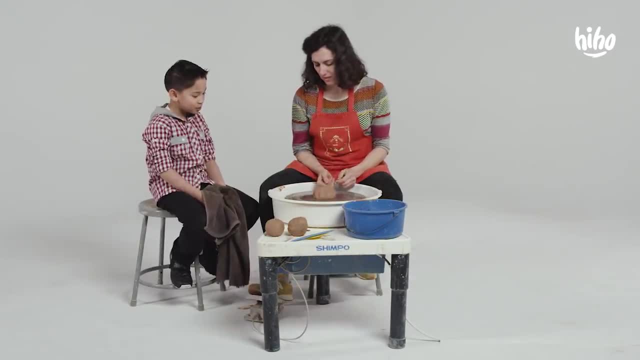 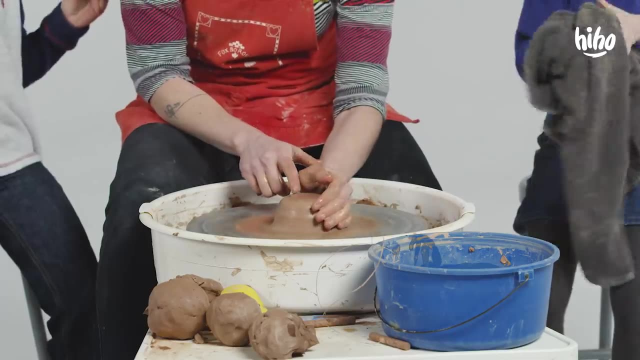 Okay, I want the clay to stick to the wheel, So I stick it on like that. How do you make a doll? I'll show you. I'll make a pot that looks like a doll. How about that? Yeah, Okay. 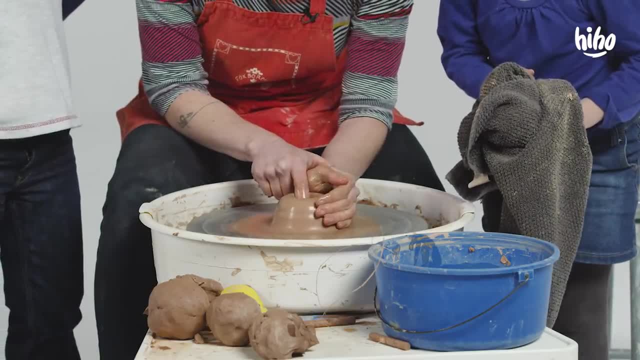 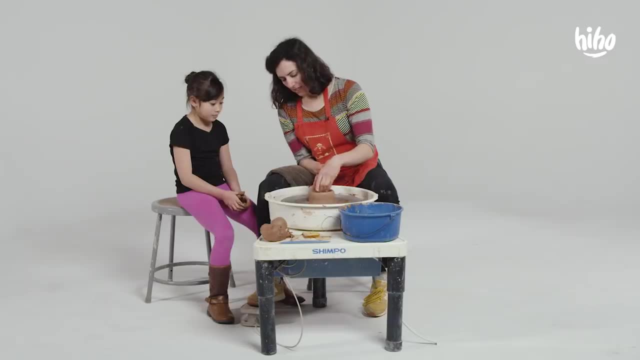 So I'm putting one hand on the outside and I'm gonna curl my finger right into the middle. Oh, that looks cool. So now I'm gonna cross my hands together and make a butterfly, and I put one hand on the outside and one hand on the inside. 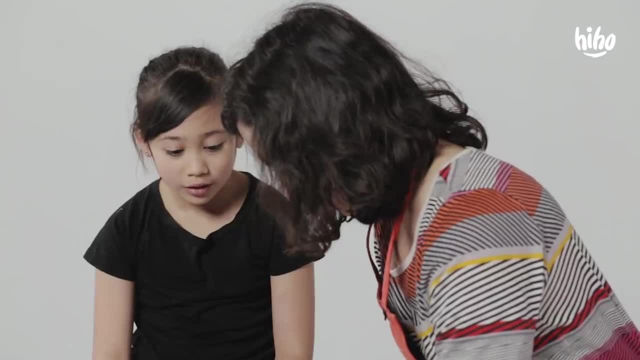 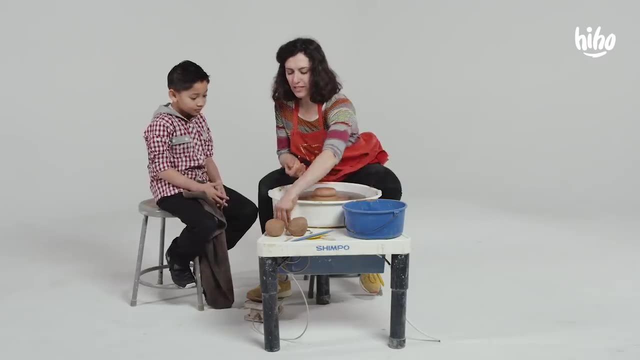 and I start pulling up with both of my hands together. Why are you so good at this? I've been practicing it for a very long time. I went to school for it. I studied it in college. I never went to college, because I'm just a little kid right now. 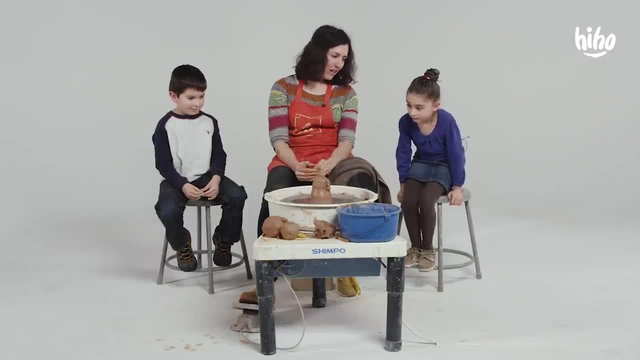 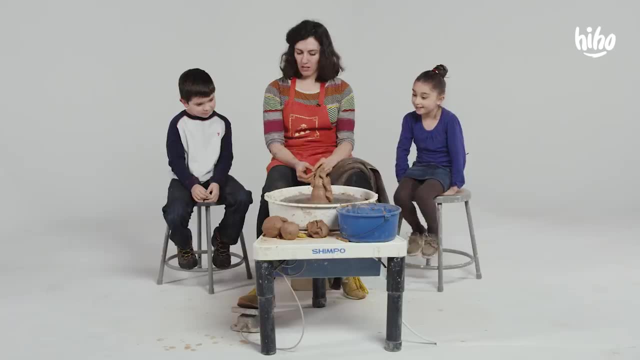 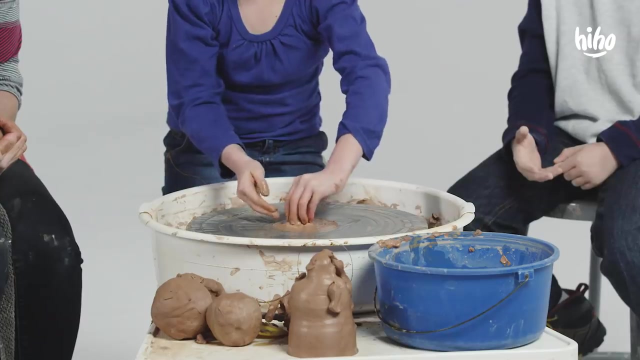 Yeah, yeah, In second grade. So what do you think? Does this look like a good doll? Yeah, we need the hair. There we go. What should her name be? Rapunzel? My turn to make it. I need help. 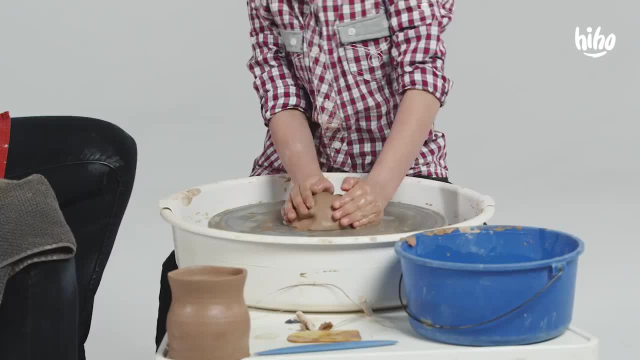 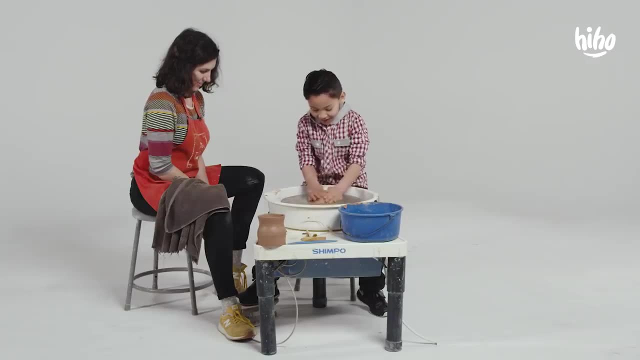 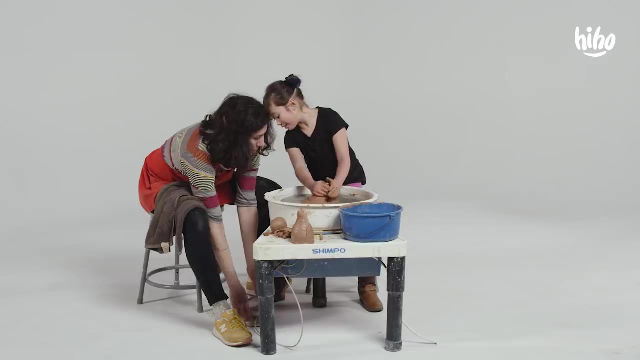 Maybe we should try with a little bit bigger. Okay, This is very fast. It's turning into like an omelet Here. I'll slow it down a little. This is not working so good. Can you help me please? 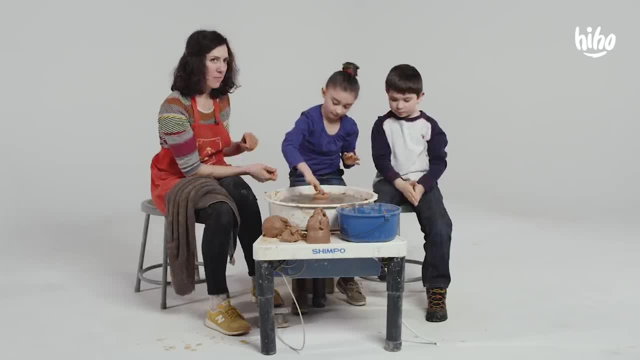 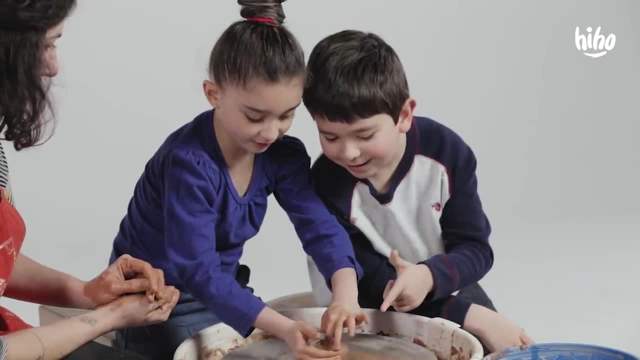 So you wanna push your finger into it, You gotta push pretty hard. I feel like I'm dipping my hand in poop. I don't know what it feels like, Because it's soupy Soupy. It feels like a wormhole pulling my finger into doom. 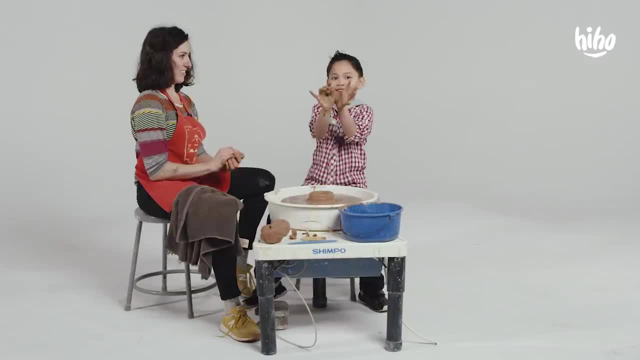 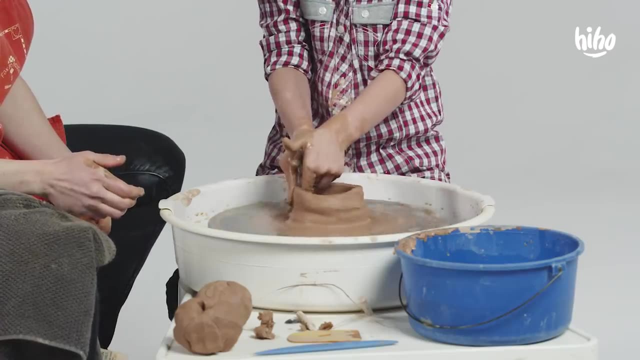 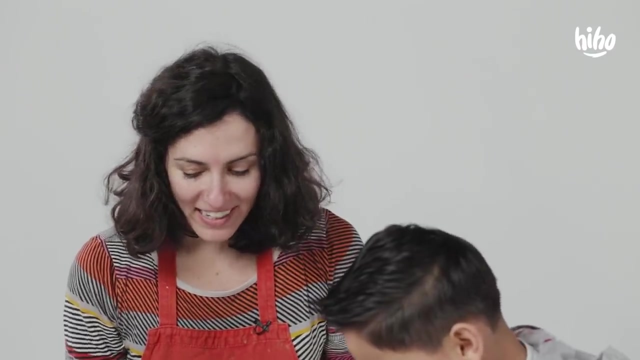 Are you scared? No, I know I won't fall in The butterfly. It got a little more up. Yeah, it is. It's getting taller. Yes, Oh No, The nice thing about clay is that You can rebuild it. 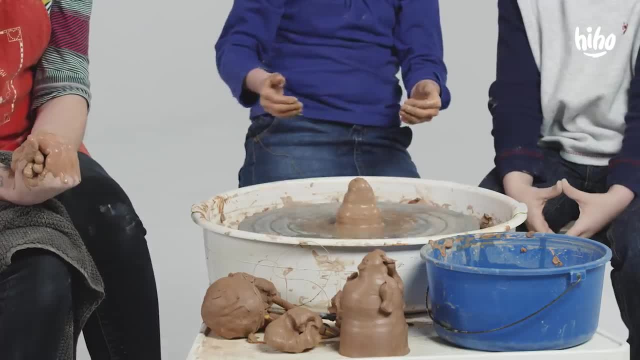 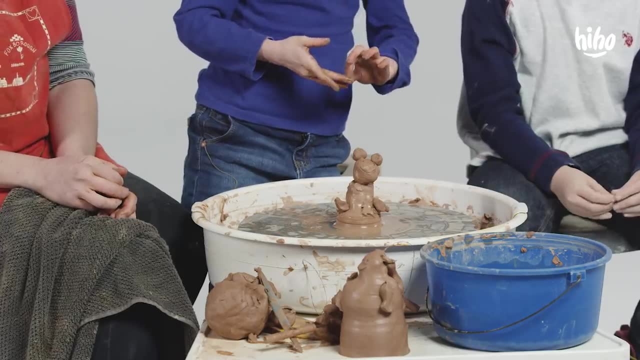 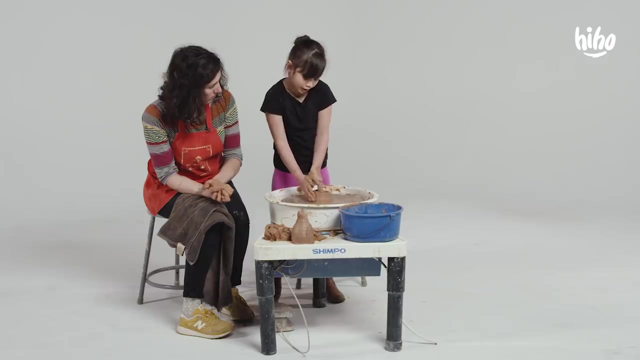 Exactly Done. That looks great. What'd you make? A doll dress, Ta-da Bon-bon. Good job, Thank you. I can't wait to see yours. Aww, I'm planning on turning it into a vase for my mom. 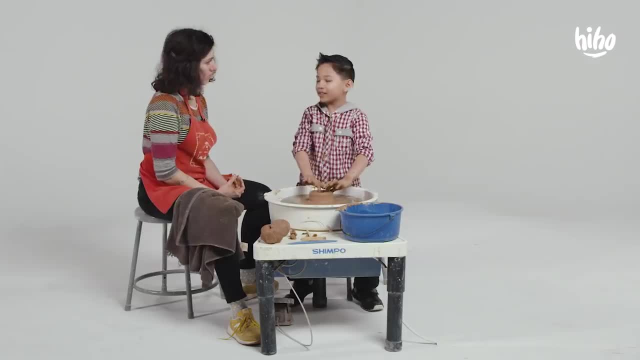 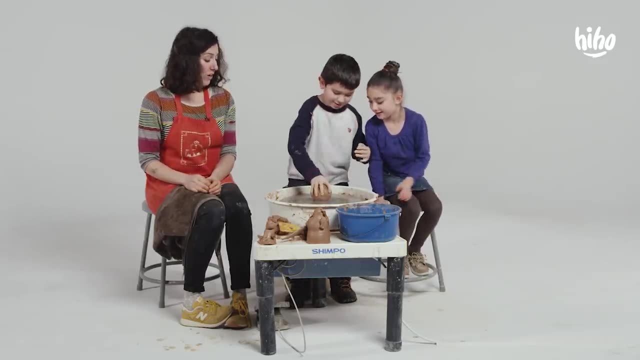 Oh, that's nice. Actually, can you make cups out of these Mm-hmm? Yes, then I'm making a cup, You're making a cup. So what are you gonna make? Not telling you? It's supposed to be a surprise. 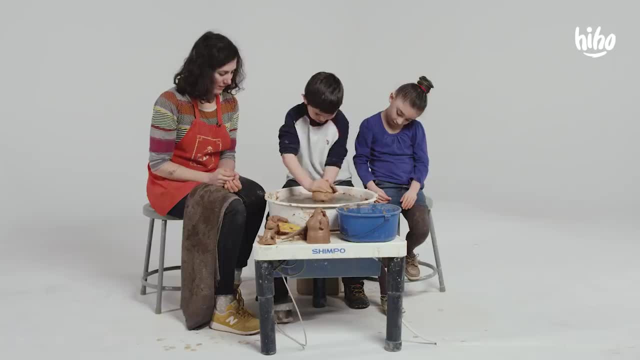 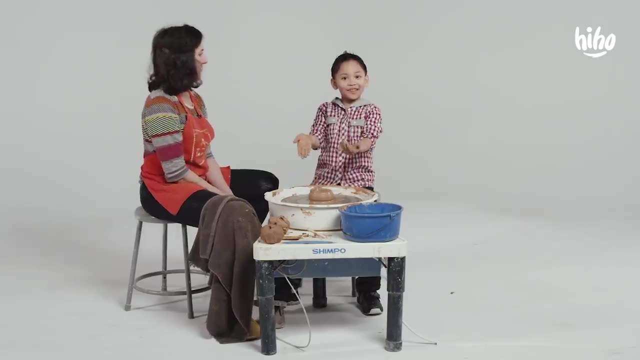 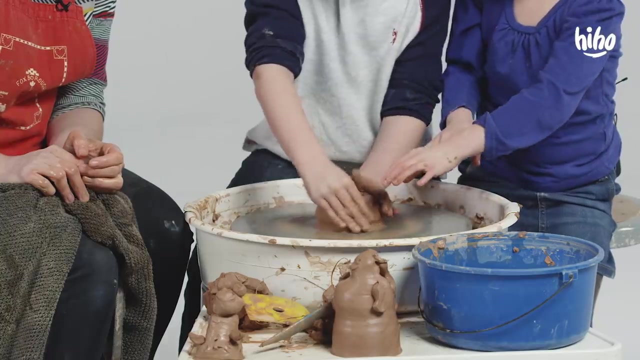 Oh, okay, How's it feel Wavy? Yeah, that's great. Can you see this, Because it actually looks so good. Okay, stop for a minute. Too fast, That's what I want. Are you gonna make a teapot? 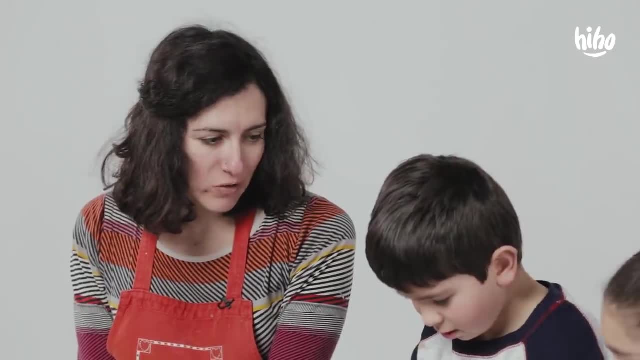 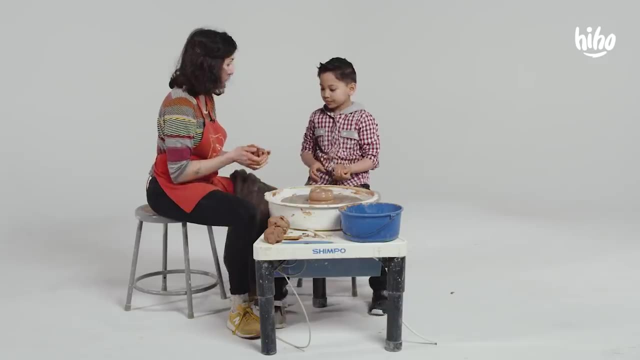 No, A dragon, No. So are you just exploring how it feels right now? I don't know what I'm making, I'm just doing what I'm doing. So you wanna make it into a handle, right? So you just roll it between your hands like that. 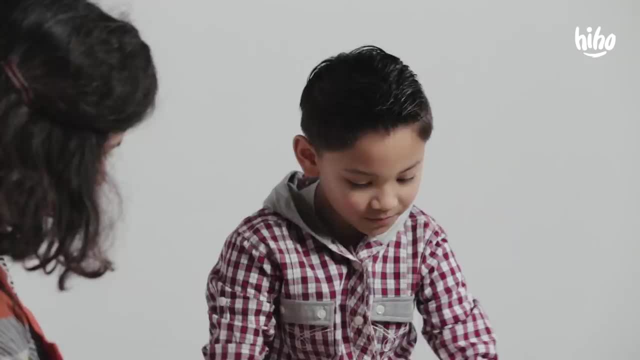 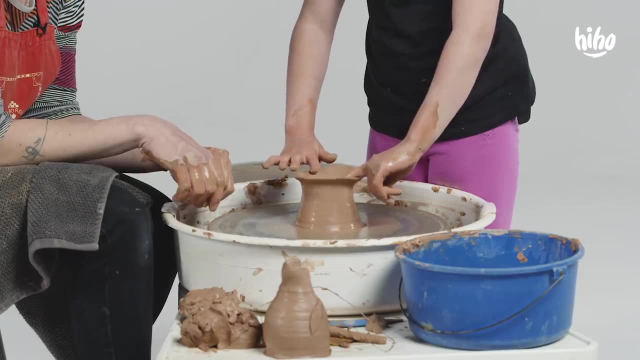 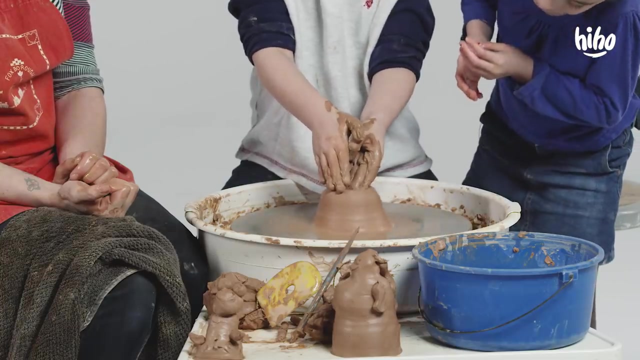 Good Yeah, Yes, I'm just doing the little wider at both sides. Okay, that's a good idea. Yeah, Butterfly, Yeah, Mm-hmm, Let's see there, Do we get up? It's making it bigger too. 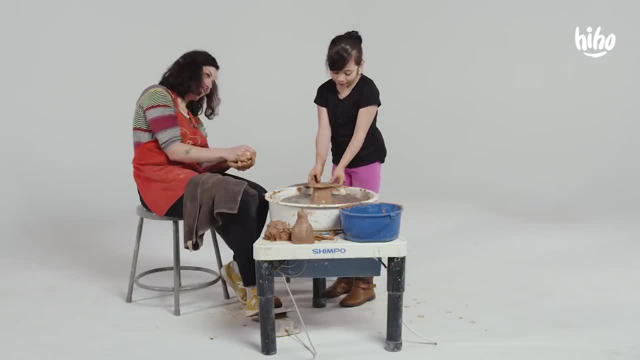 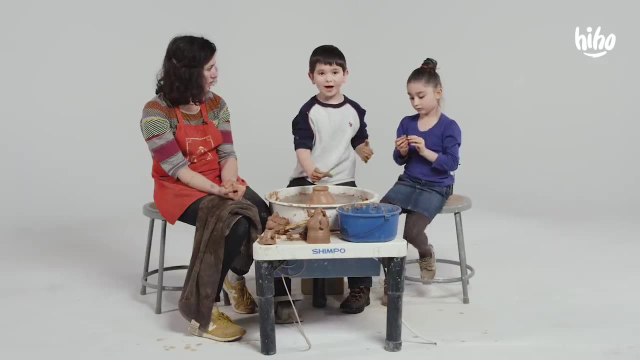 It is. It's really cute. now It is cute. It looks like an upside-down top hat. Oh, I never actually thought of it that way. I could put flowers in it. I could chuck my Legos inside of it. I can mostly do anything with it.